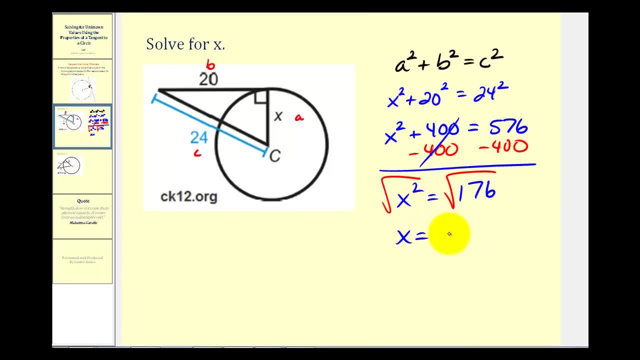 So we have: x equals the square root of one hundred seventy-six. Now we should try to simplify this. So let's go ahead and see if we can identify any perfect square factors of one hundred seventy-six. This number is divisible by four. One hundred seventy-six is four times forty-four. 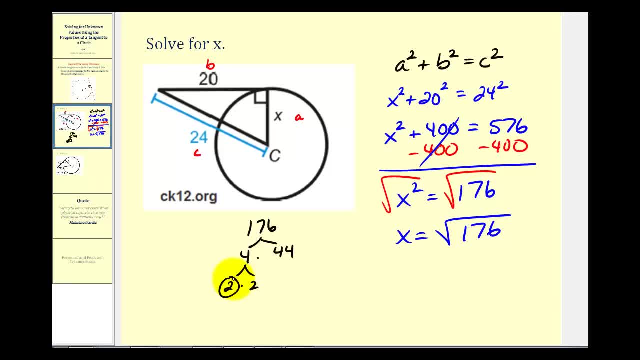 Four is equal to two times two, which are both prime. Forty-four is four times eleven, Eleven is prime, and then four is again two times two. So we want to show some work here. We have: x equals the square root of. we have four factors of two. 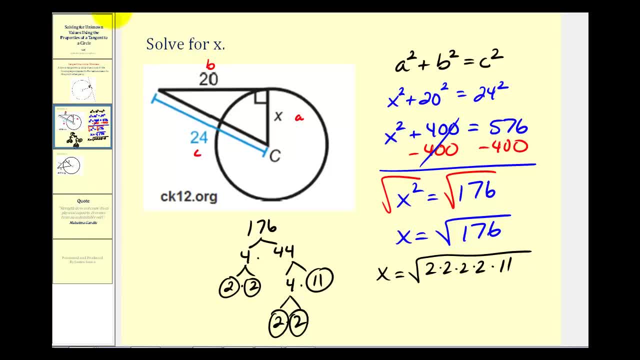 and a factor of eleven. Every time we have two equal factors, we have a perfect square factor. So two times two is four, that's a perfect square. Two times two is four, that's a perfect square. So this pair gives us a two. this pair gives us a two. 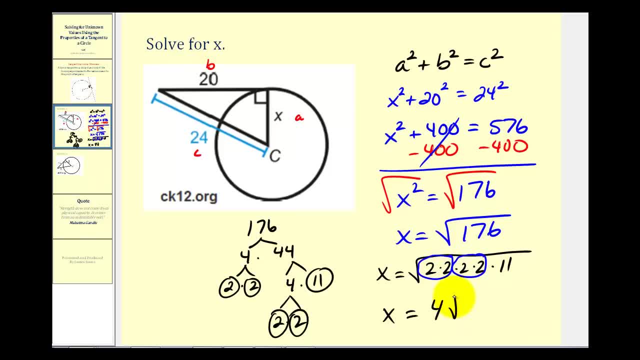 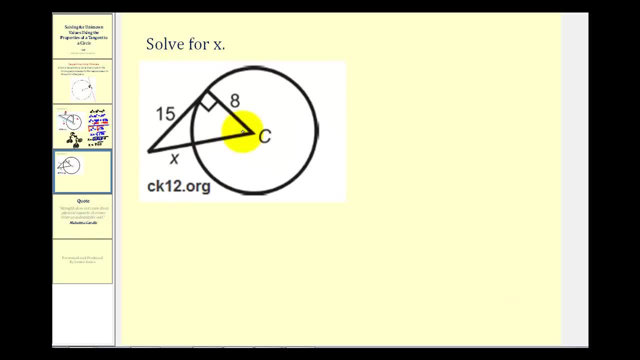 So we have a four outside the square root, So four times the square root of eleven. Now let's take a look at our second example. Again, it's the same type of problem. Here we're given a tangent segment and the radius of the circle drawn to the point of. 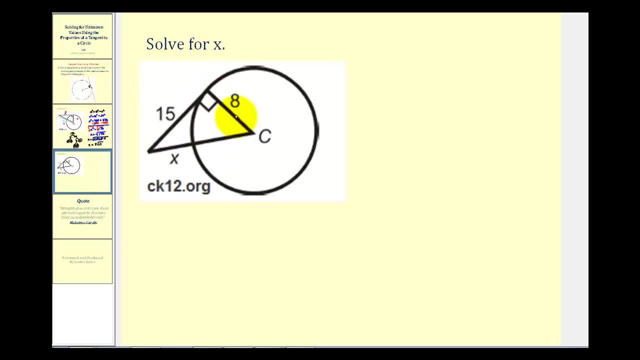 tangency. So we know we have a right angle here. So now that we have a right triangle, we can use the Pythagorean Theorem to determine the value of x. But notice how now we're going to be solving for the hypotenuse. So this will be side c. 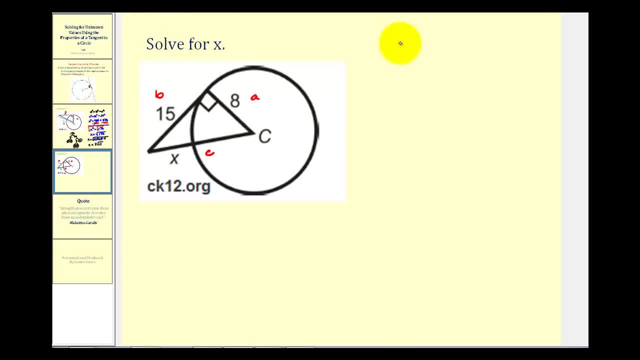 And we'll call this side a and this side b. So again the Pythagorean Theorem. we have: a squared plus b squared equals c squared. So now we're going to have eight squared plus fifteen squared equals x squared. Well, eight squared. 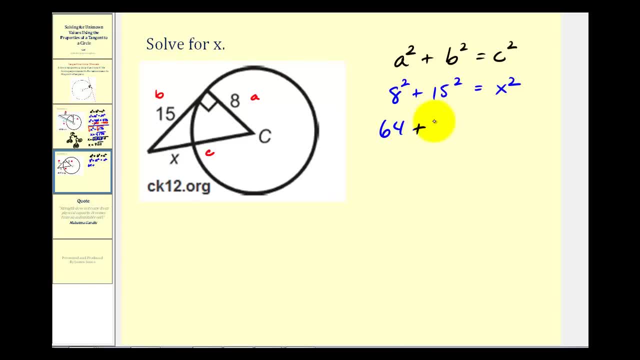 is equal to sixty-four. Fifteen squared is equal to two hundred twenty-five. Sixty-four plus two twenty-five equals two hundred eighty-nine. And again we're going to take the square root of both sides And because it's a length on a triangle,